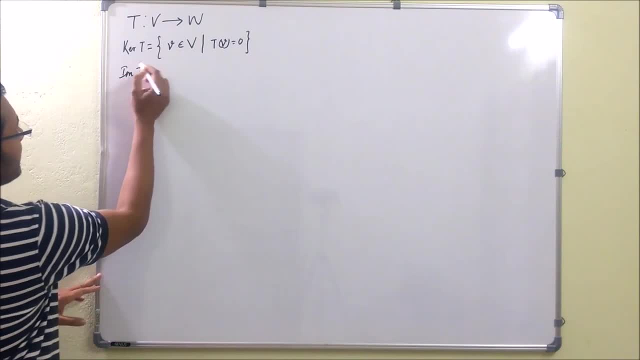 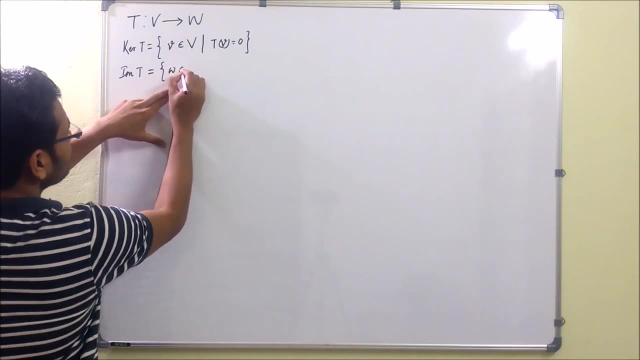 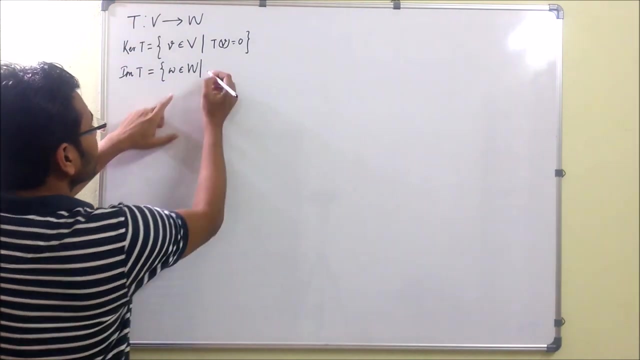 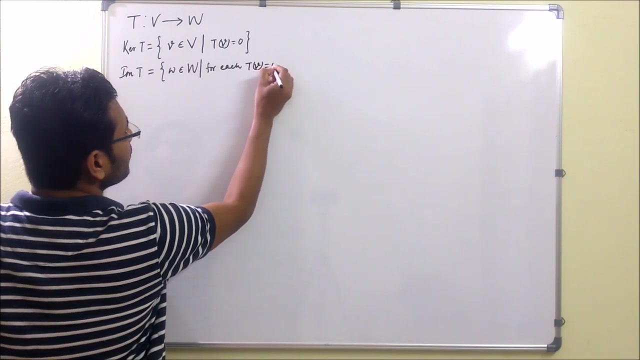 Now what is image of T? So we write image of T as imt this. So this is nothing but the elements. W belongs to this W vector space range set such that for each T of V equal to W where V belongs to this V. 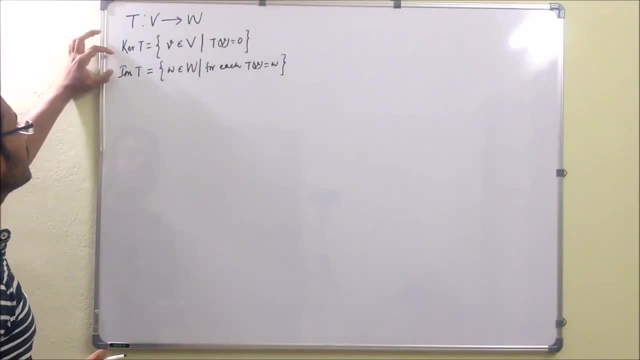 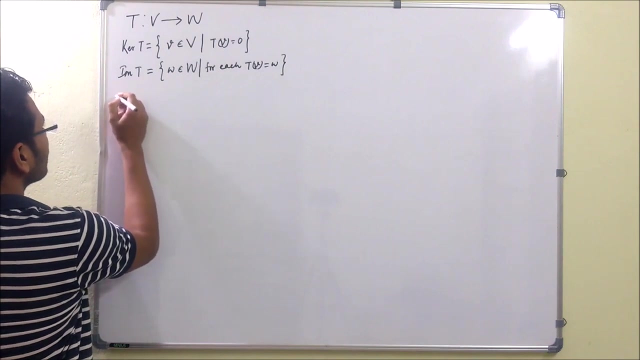 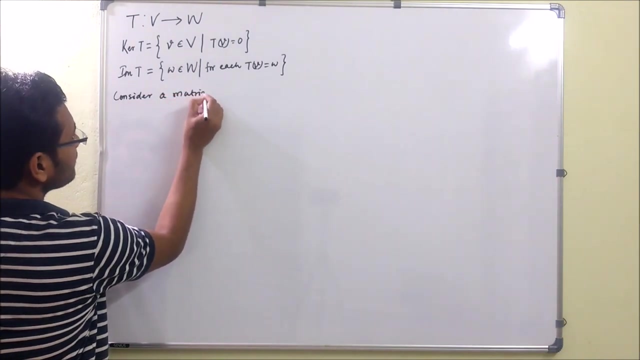 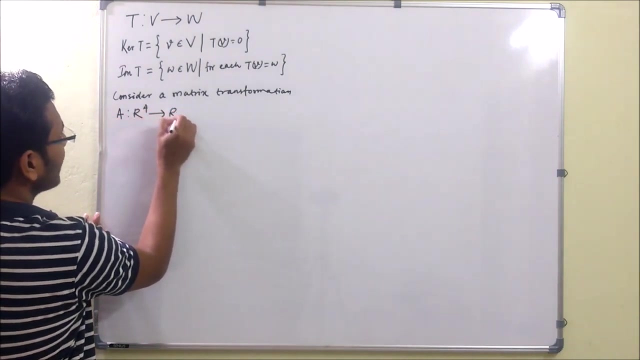 So in this way we can define, to set. these are kernel of T and image of T. Now we will take one example and we will see the dimension basis of this. So we have to consider a matrix transformation, That is, A from R4 to R3.. 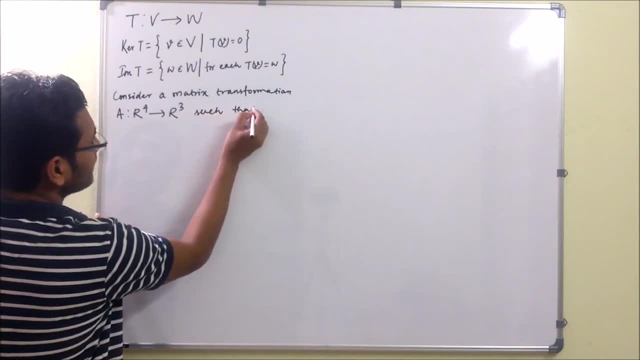 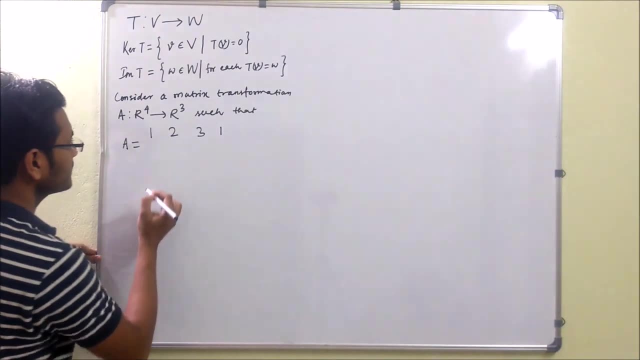 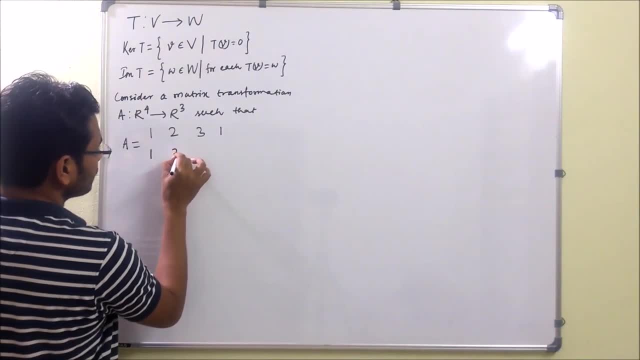 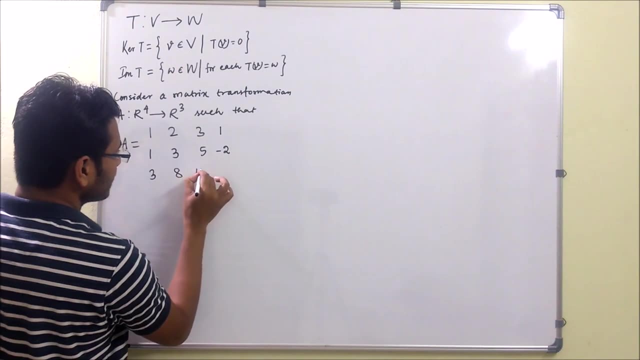 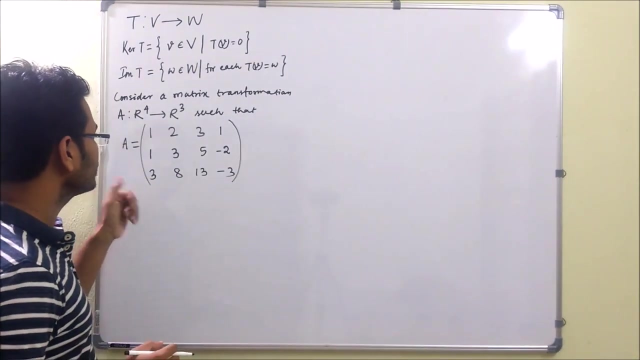 Second row is 1,, 3,, 5, minus 2.. And third row is 3,, 8,, 13, minus 3.. So this is the transformation matrix And, using that, what we have to find, We have to find. 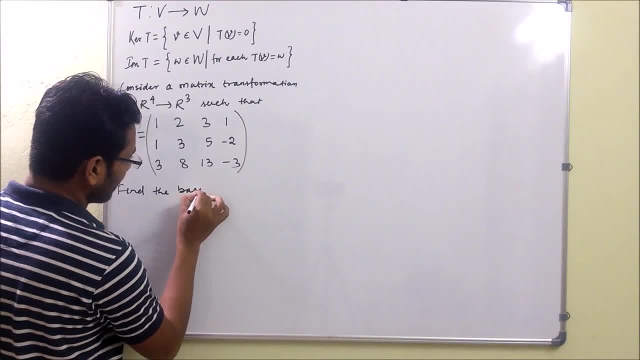 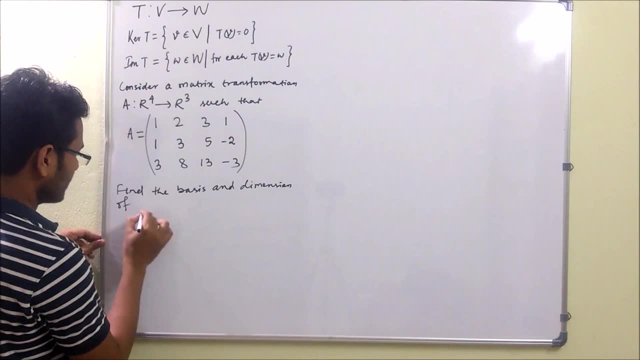 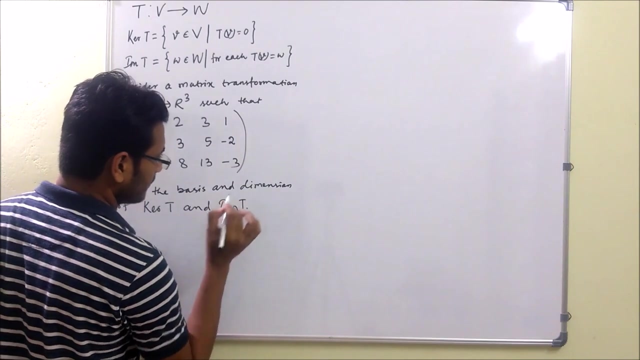 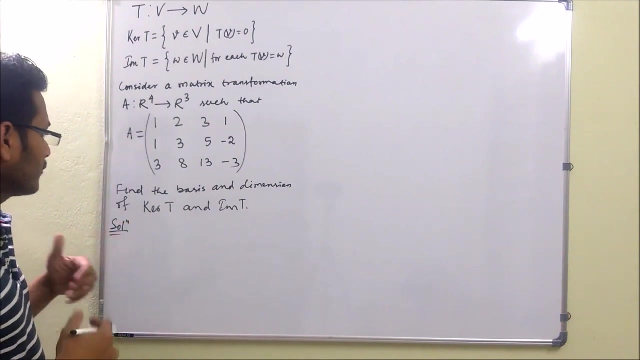 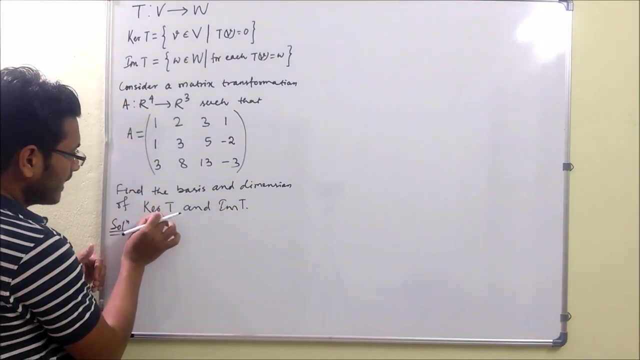 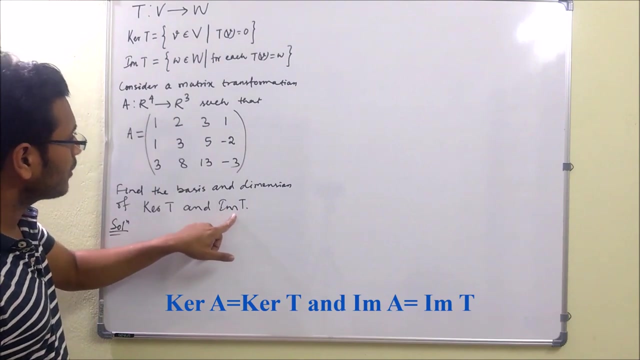 The basis and dimension of kernel T and image of T, So that we have to find, So we have to do the solution. Now, how to find, How to do the solution that we have to see. We see that kernel of T, The elements of kernel of T, belongs to V and elements of image of T belongs to W. 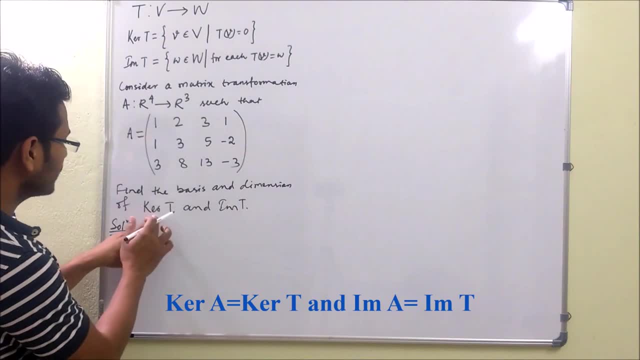 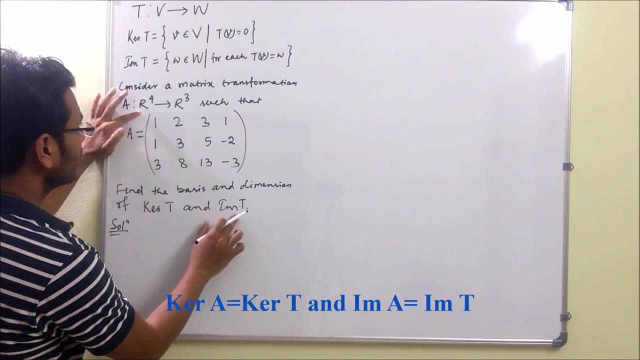 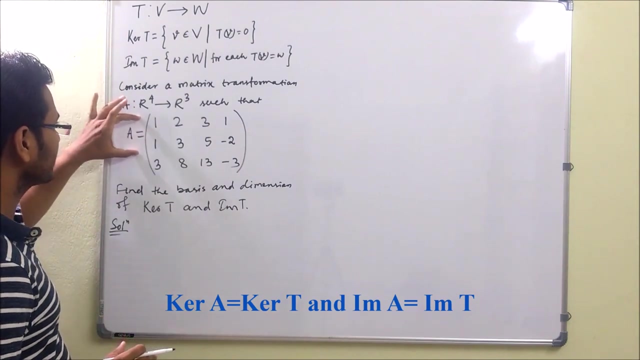 That means here, if we see the transformation kernel of T, all the elements of kernel of T will belongs to R4.. All the elements of image T will belongs to R3.. So now, to find the kernel of T, we have to start with this matrix and we have to see: 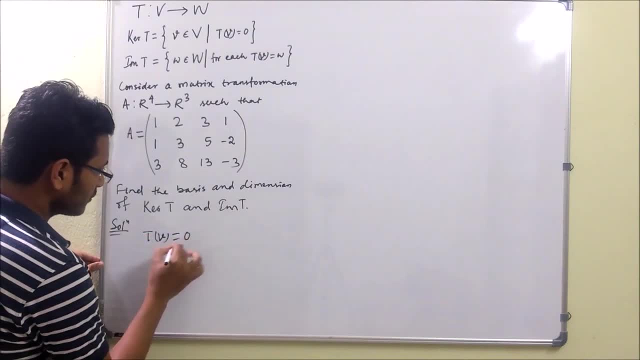 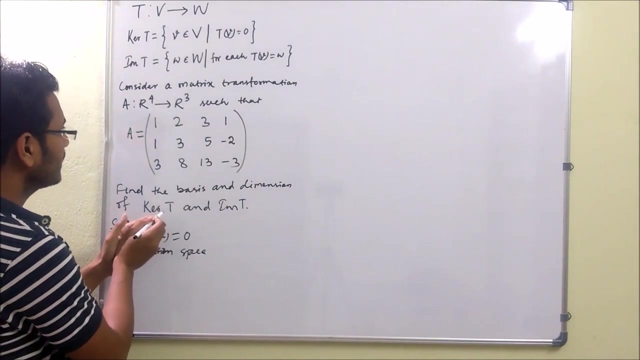 the solution T of V equal to 0.. So we have to see the solution space Solution: space of T of V equal to 0. And we see that here the kernel of T, the vector, will be R4.. Will be in R4.. 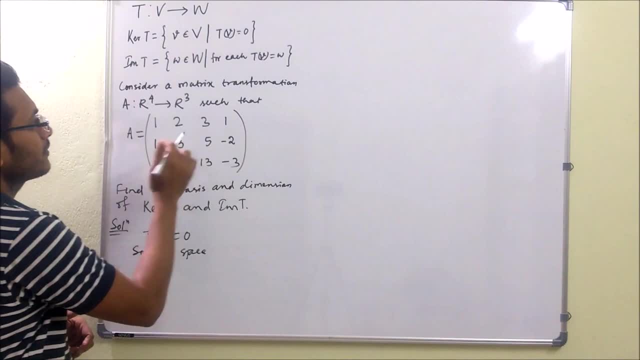 There will be 4 components. So we will start with this matrix And we will see row wise operand. So we will start with this matrix And we will see row wise operand And we will see R4.. So we have to start with this matrix. 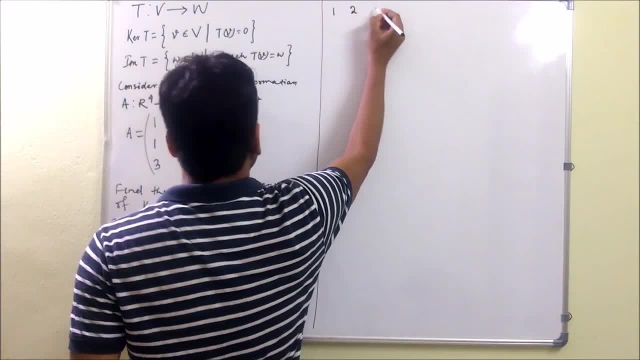 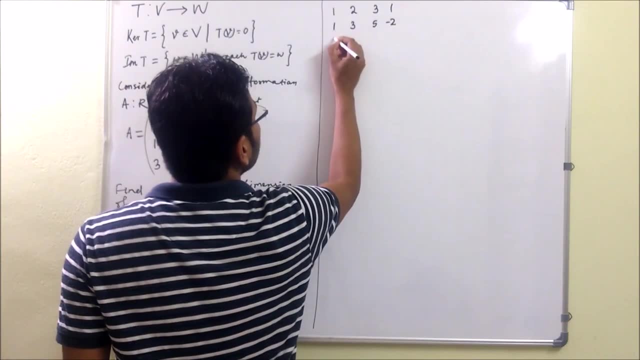 And then we will write our simple operation and we will see what will happen. So we will write the matrix, that is 1,2,3,1,, 1,3,5,-2,, then 3,8,13,-3.. 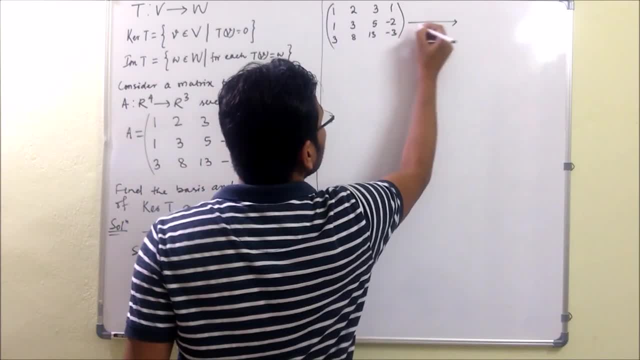 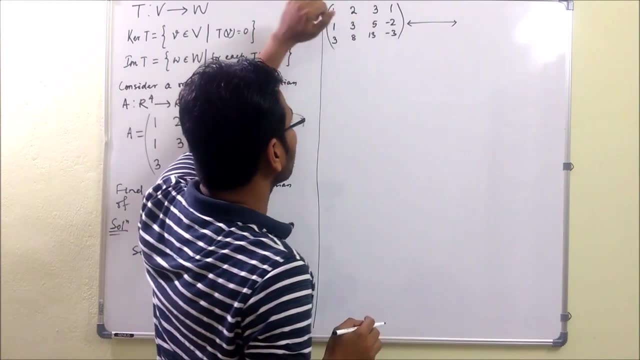 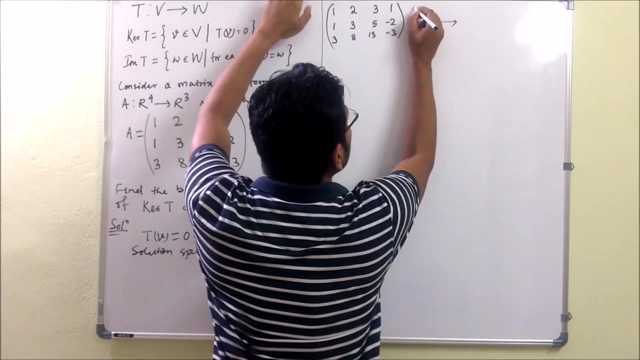 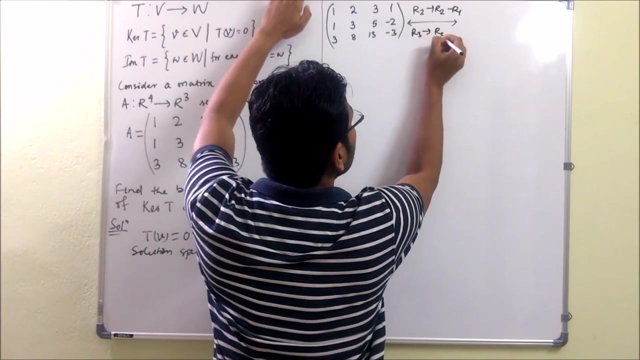 Now what to do? We have to apply Gauss Elimination Rule and we have to convert this matrix to row echelon form. So what to do? We have to make these two entries, 2 and 3,, 0.. So how to do So? row 2 will be row 2 minus row 1 and row 3 will be row 3 minus 3 or 1.. 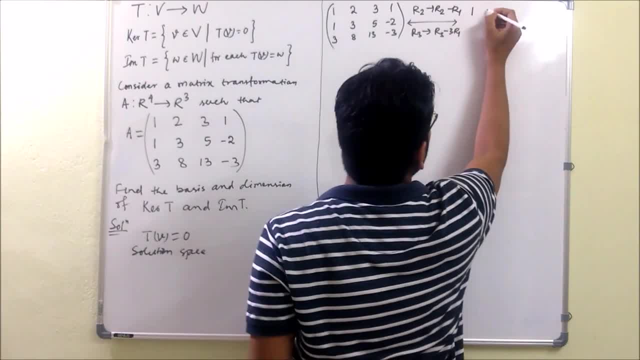 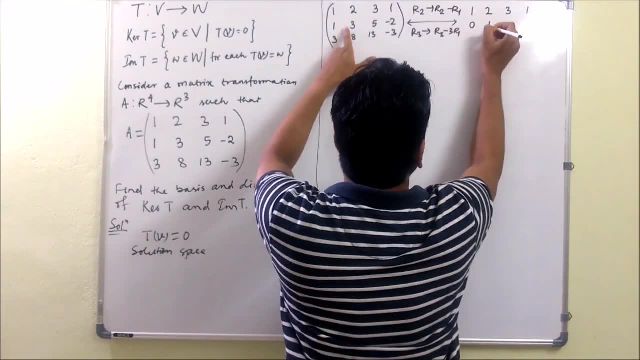 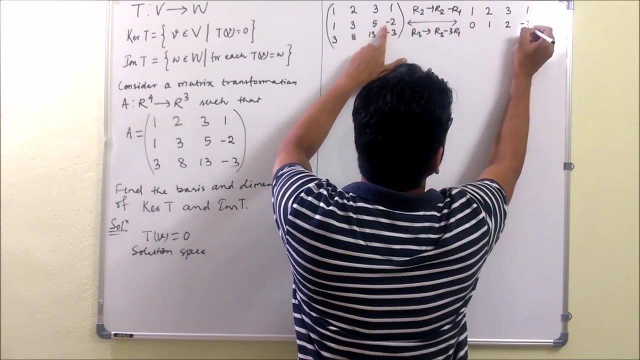 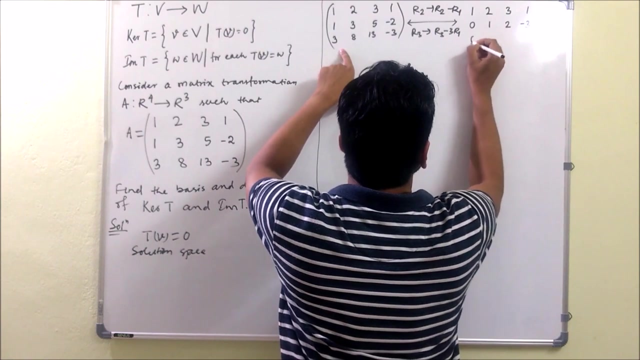 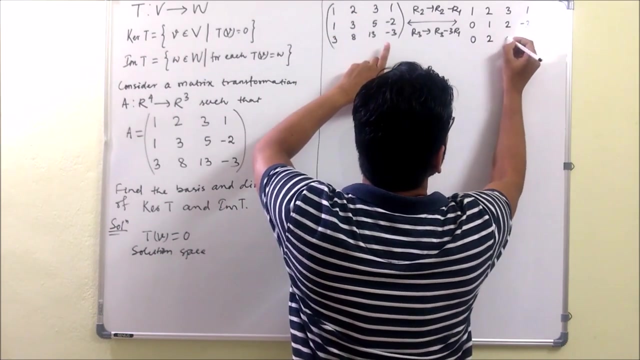 Then it will be 0.. So first row will be same: 1, 2, 3, 1.. Second row will be this one: 0, 3 minus 2, 1, 5 minus 3, 2, minus 2, minus 1, minus 3.. Now this one: 3, minus 3, 0, 8, minus 6, 2, 13 minus 9. 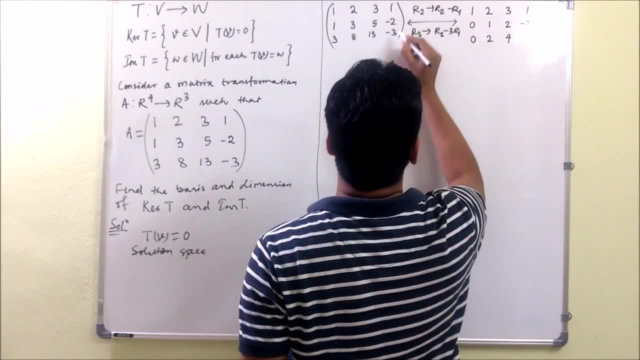 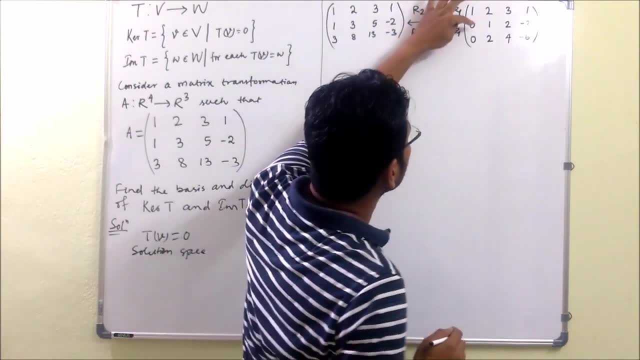 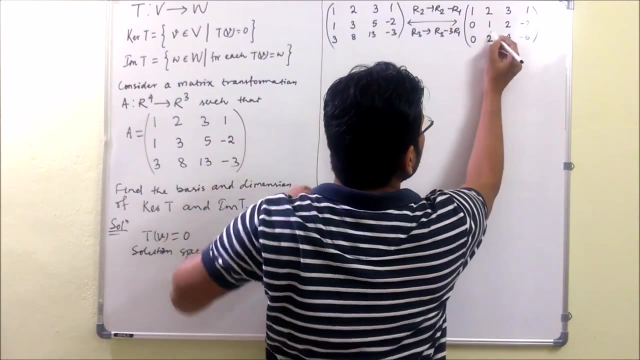 will be 4.. Now minus 3, minus 3, minus 6.. So now what will happen If we see? then we can see that this is 1, 2, minus 3 and this is 2, 4, minus 6.. So if we want to make this element 0,, 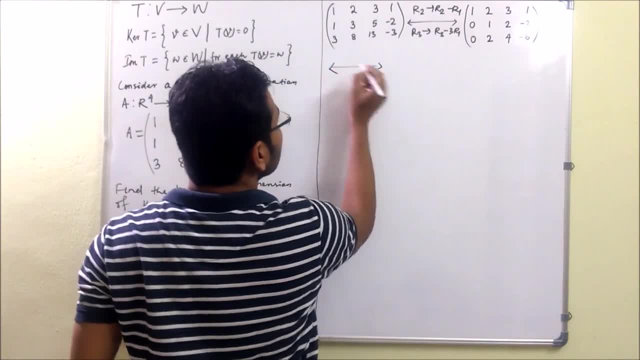 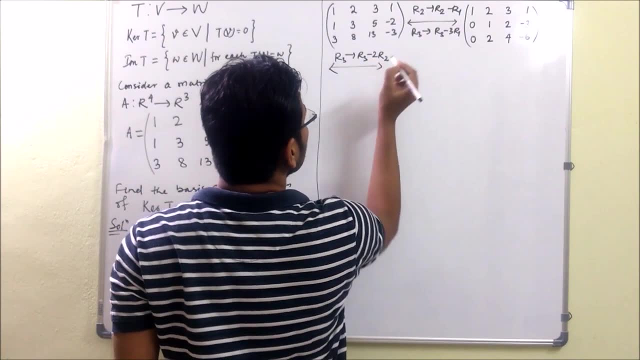 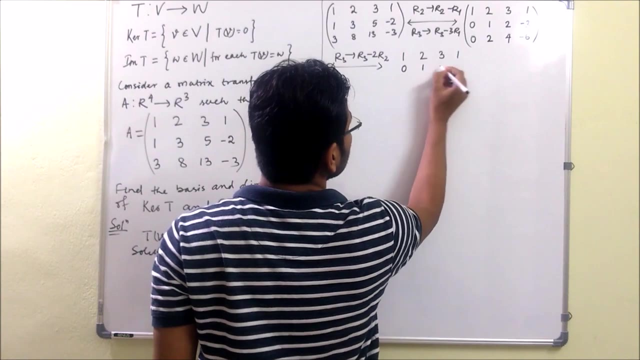 what to do. We have to write what R3 changes to R3 minus 2 R2.. So if we do like that, then first row will be unchanged, second row will also unchanged and third row will be this two: 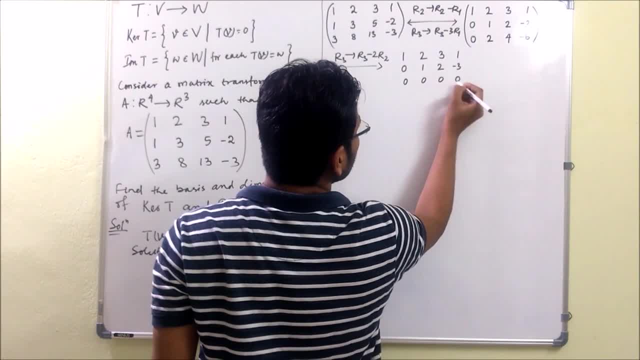 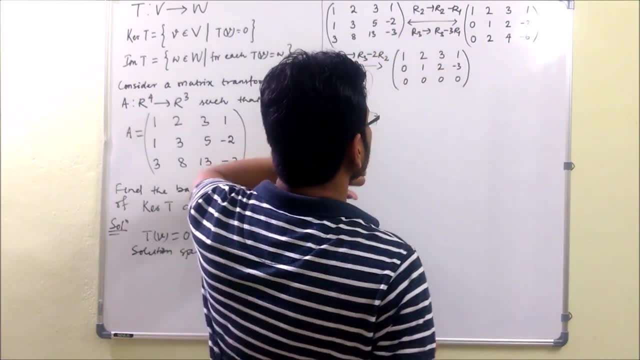 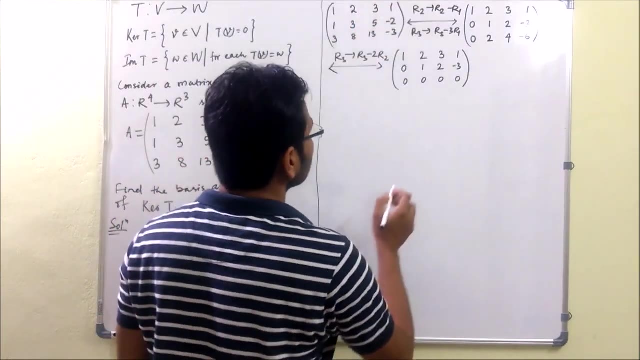 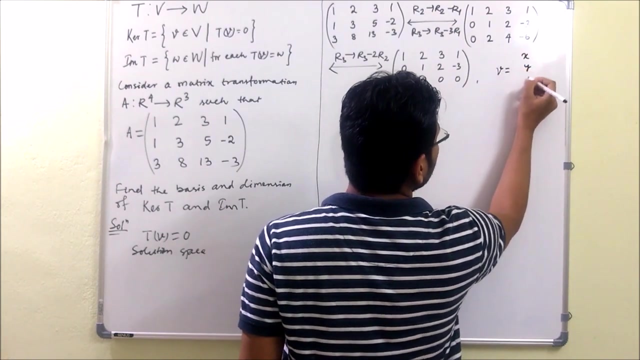 minus 2, 0.. So all the elements of the last row will be 0,. that you will get Now. this is the form. Now what happens Here? we can see that if, for each component, if we mention, if we write the vector v as x, y, z, t, so then what will happen from this? 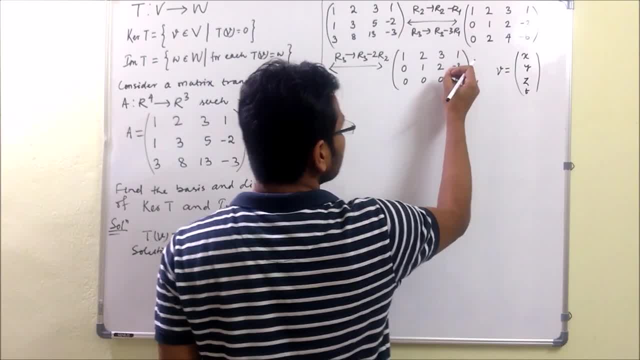 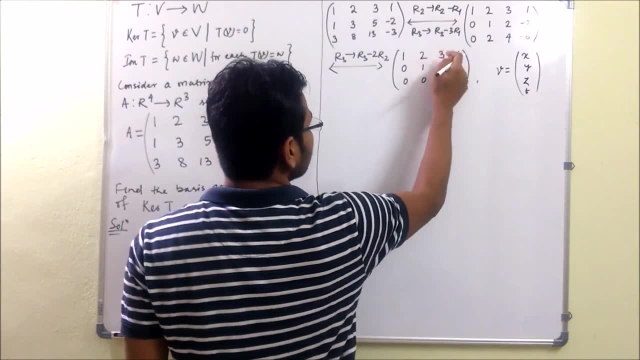 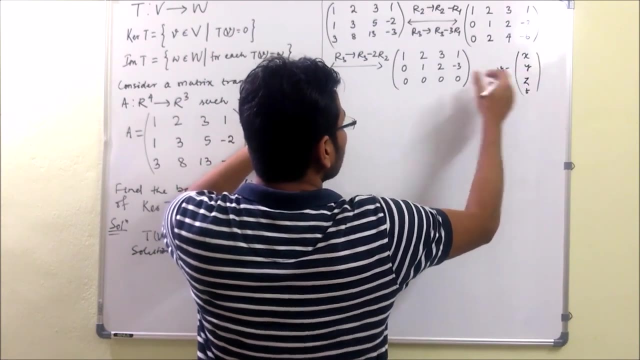 How to get. So this is solution equation, solution: space. So from these two equation you can find, because last equation is 0.. So last second equation is what, If we write in terms of: if we multiply this with this, okay, because this into this will be 0, that will be solution. 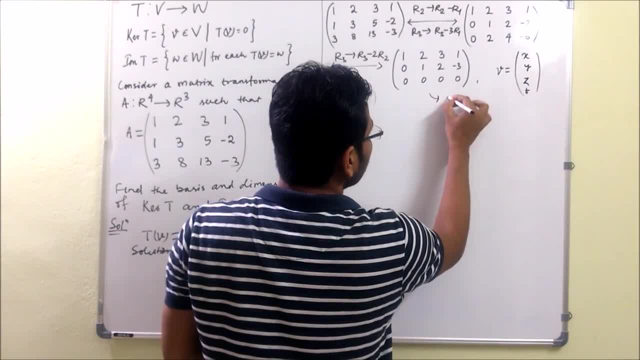 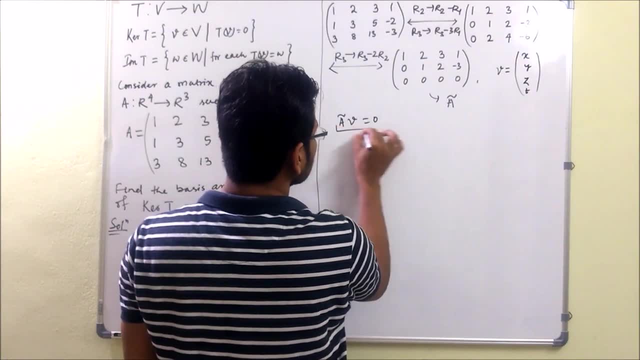 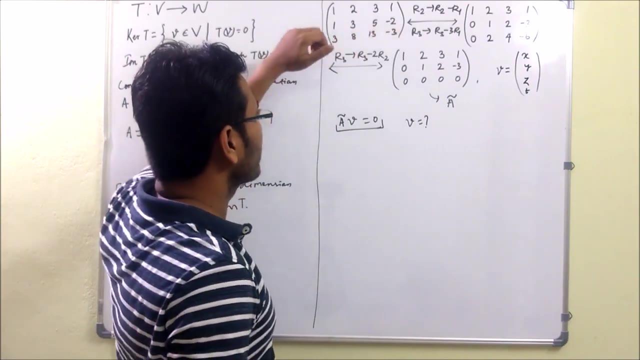 space. If I write this as A tilde, then what will happen? A tilde, this v equal to 0,, this 0.. So solution for this, okay, solution for this will be the solution. space for this problem. 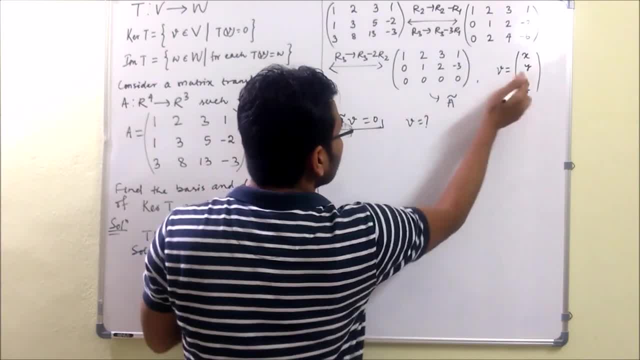 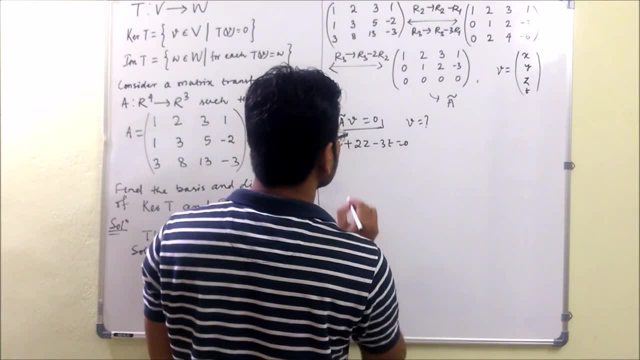 Now how to get so 1,, 2, minus 3, so if I write so, it will be y plus 2z minus 3t equal to 0, first equation. So from first equation how to get so y will be what? 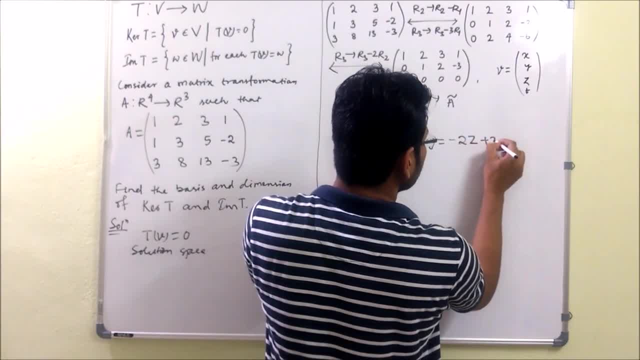 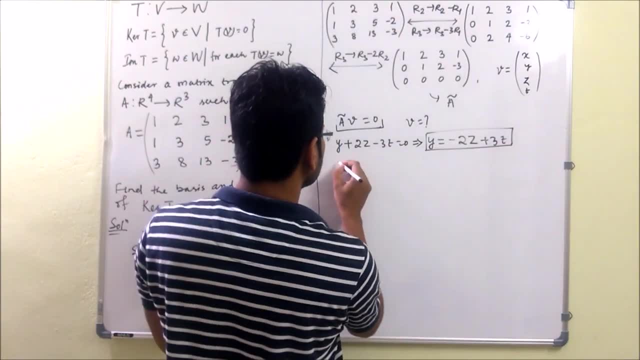 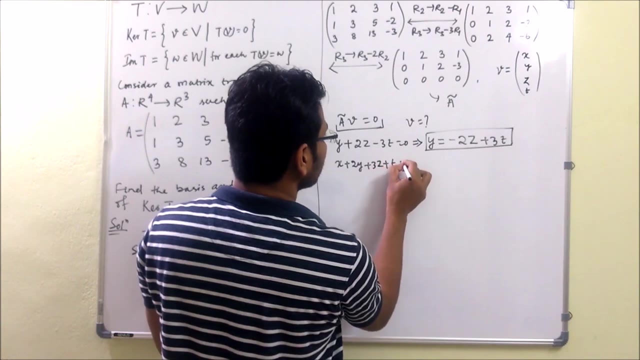 1, minus 2z plus 3t. we will get this relation Now if we put y value here in the first equation. it will be so first we will write the equation x plus 2y plus 3z plus t equal to 0. So from: 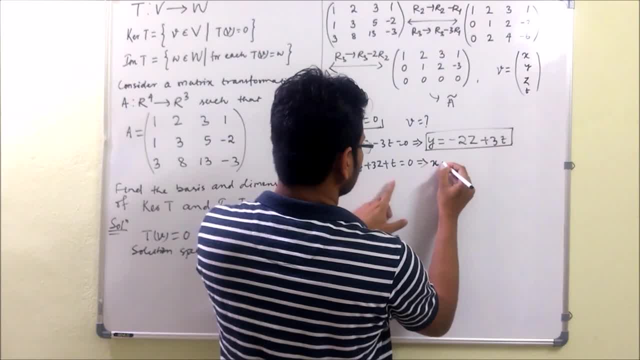 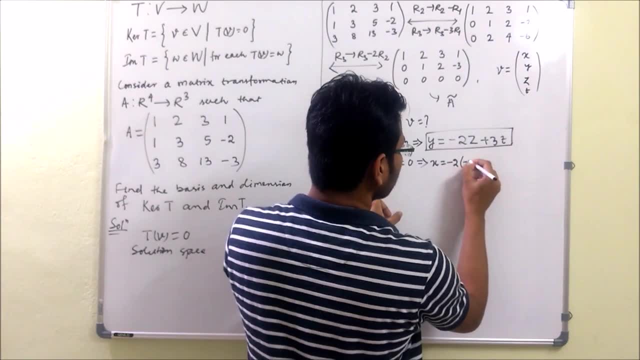 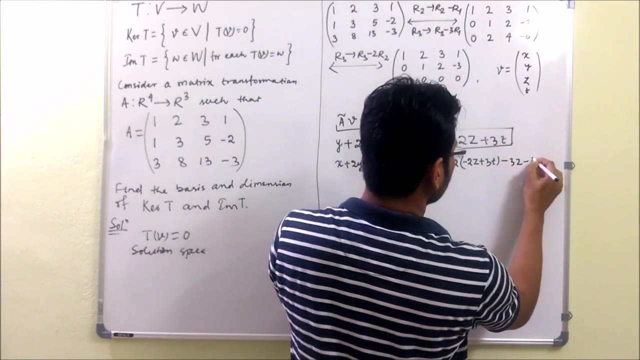 this: it will be x so x. if you take all right side, it will be minus 2 into y in place of y. you can put here This: minus 2z plus 3t, then minus 3z minus t. So if we solve, then what we will get. 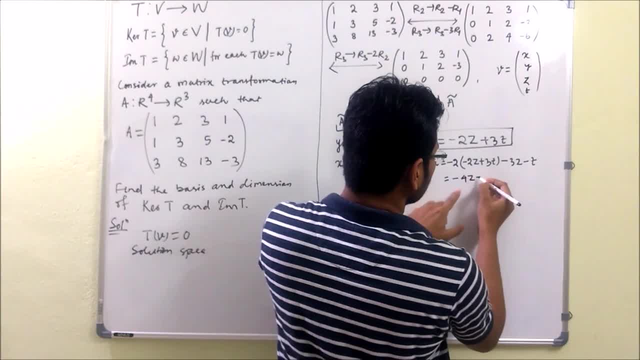 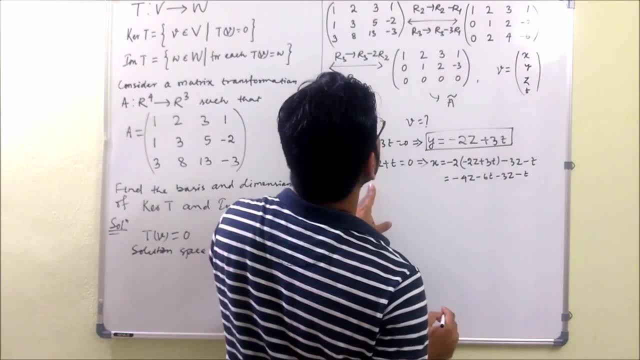 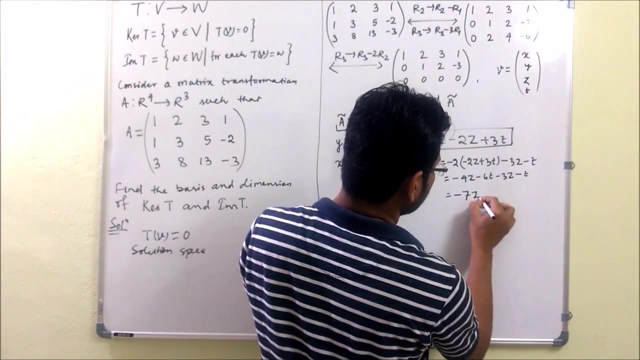 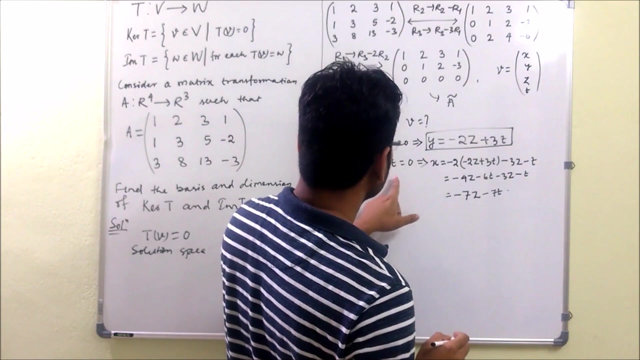 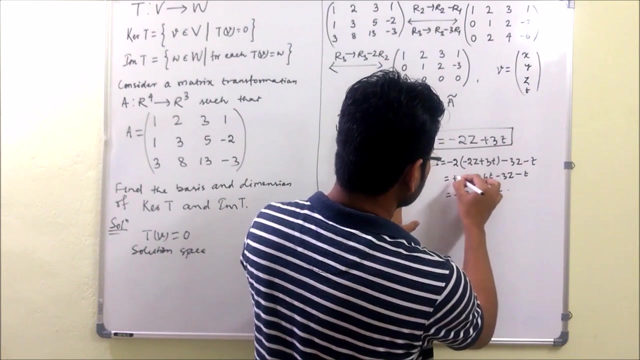 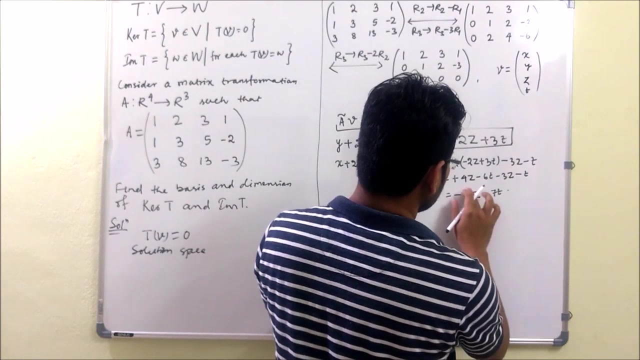 x equal to minus 4z, then minus 6t, minus 3z minus t, Whether it is correct. Okay, Then it will be minus 7z. okay, So it will be plus minus, minus, plus. this will be minus. okay, Now this will be. 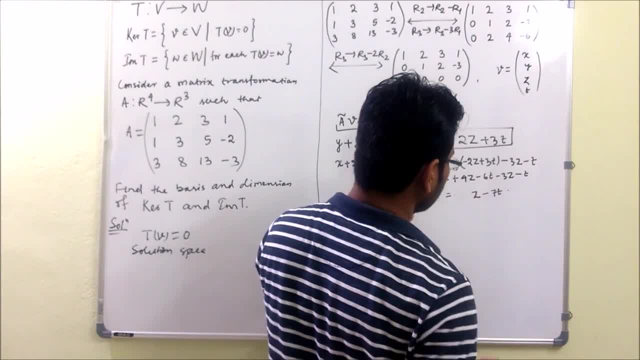 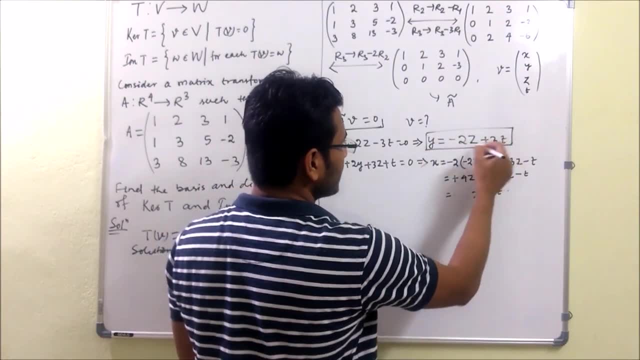 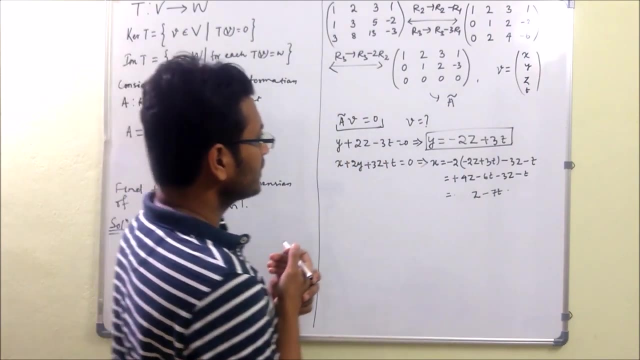 only plus z, minus 7t. Now, what we will do then? how to construct, as y depends on t and z, and x also depends on what t and z. So, in that case, what to do? We have to take. 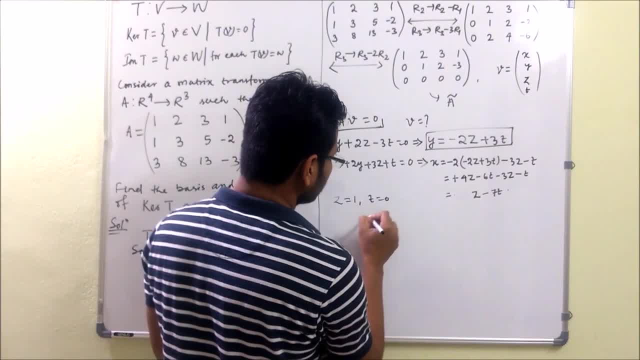 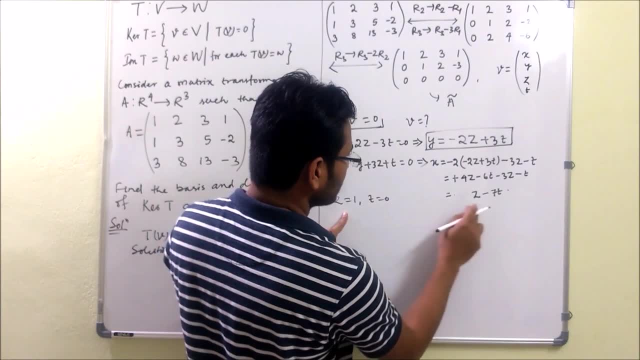 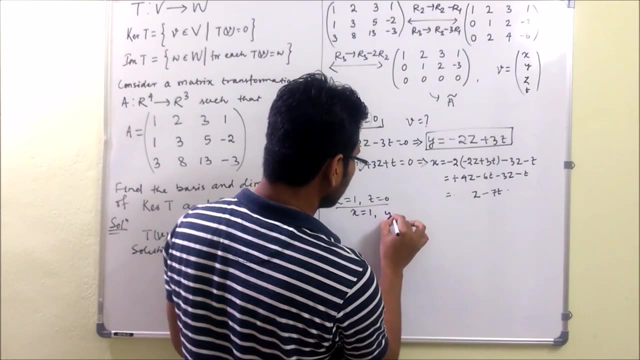 z equal to 1,, t equal to 0,, then we will get one solution. What will be the solution If we take z equal to 1,, t equal to 0, so it will be 1.. So x will be 1, and y will be. 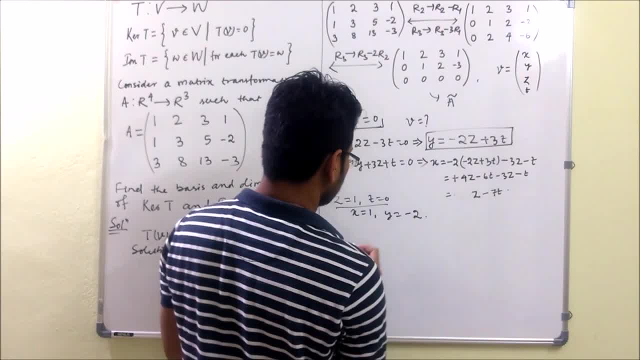 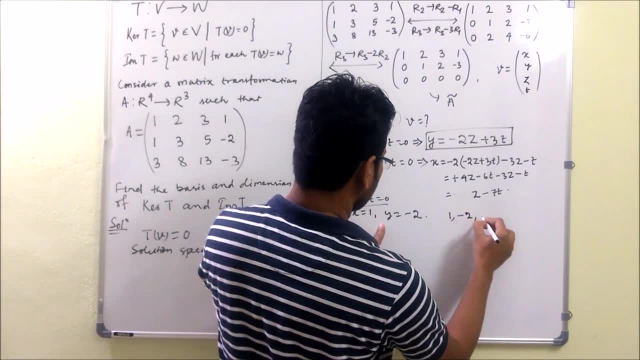 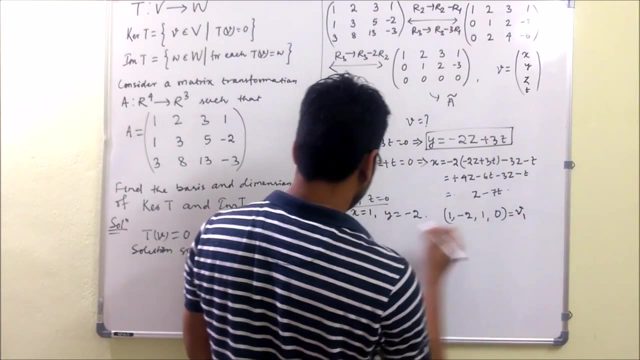 what Minus Minus, Minus, Minus Minus 2.. So this is one solution. one solution. You can write it as 1, minus 2, 1, 0.. So this is one solution. If it is v1,, then second, If I take z equal to 0 and t equal to 1,, then 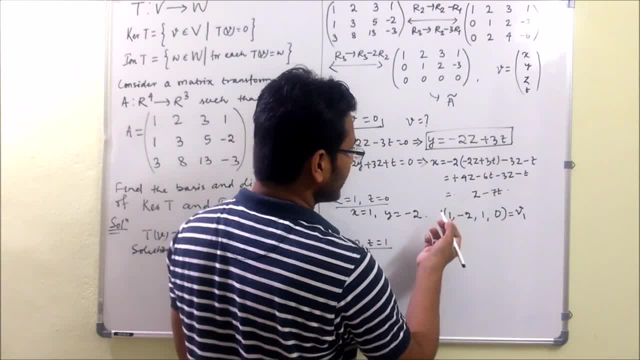 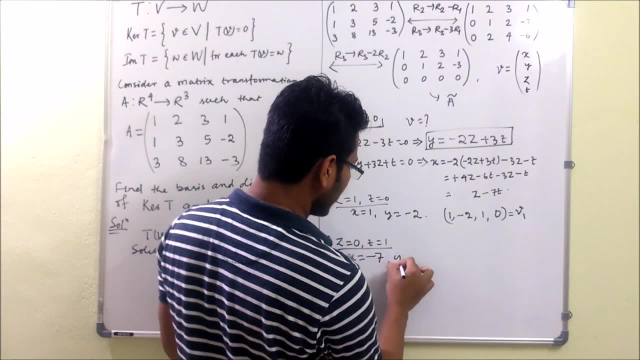 again, we will get one solution. What will be that? So we have to put here: So x will be simply minus 7. Then y will be here. if we put then z value, so it will be 3. Then what will be the solution? 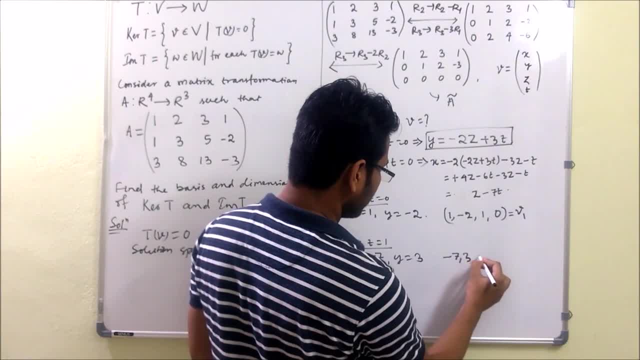 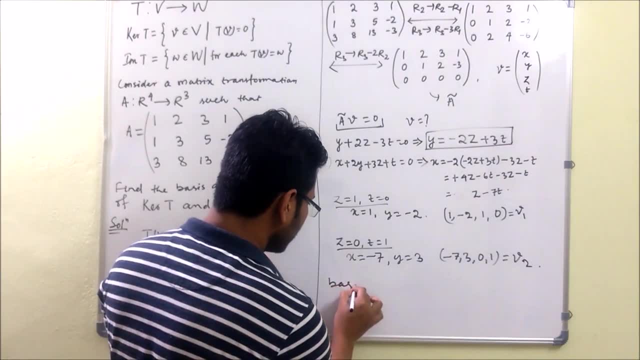 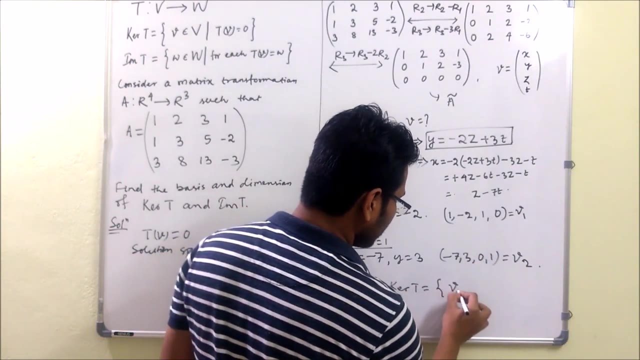 So minus 7, 3,, 0,, 1.. So this is v2.. Now, what is the basis of? Now, basis of kernel of t will be what then? This is nothing but the set v1 and v2.. Now, what is the diagonal? 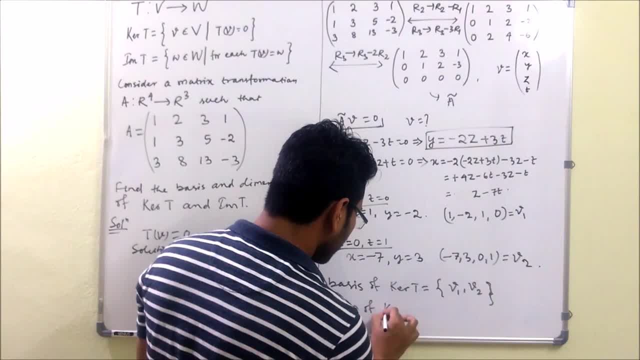 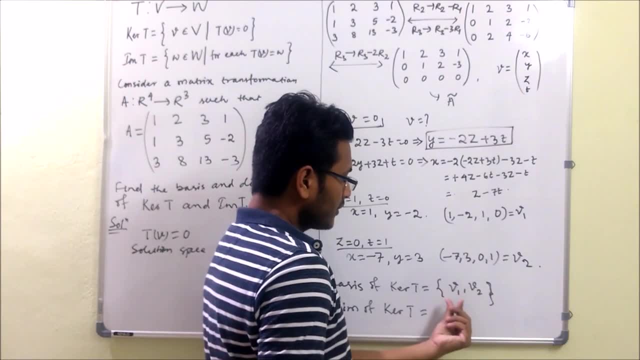 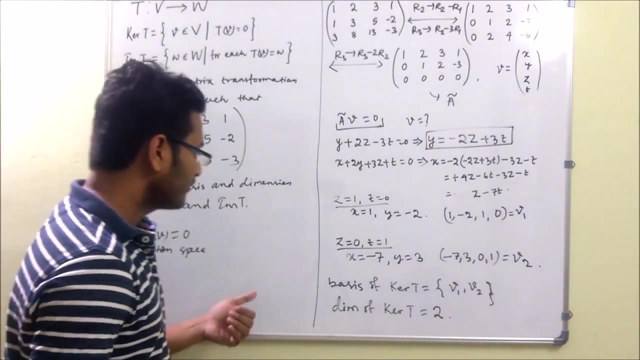 What is the dimension of this Dimension of kernel of t? So dimension is the number of vectors present in basis. So number of vectors is 2.. So dimension will be then 2.. So in this way we can find the basis and dimension of kernel of t. Now we will see. 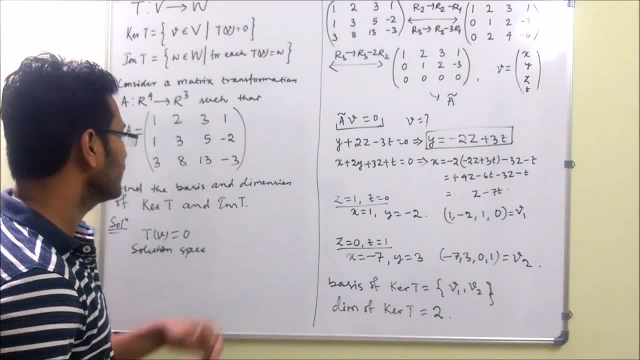 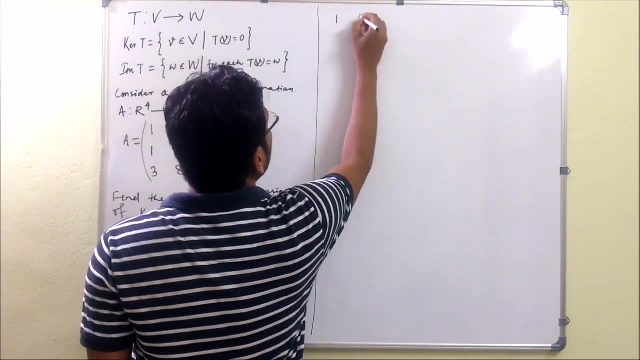 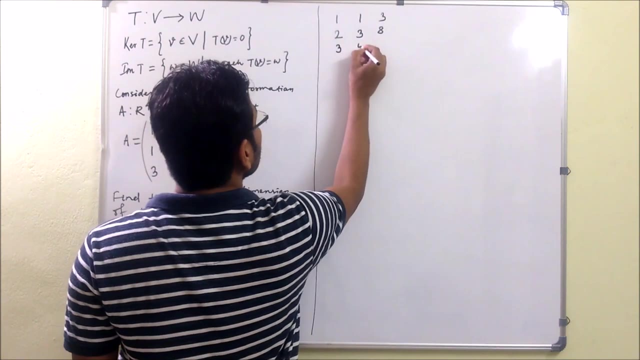 how to find the basis and dimension of image of t. So y transpose will be Here. so the first row is 1, 1, 3.. Second row: 2, 3, 8.. Third row, 3, 5, 13.. Then fourth. 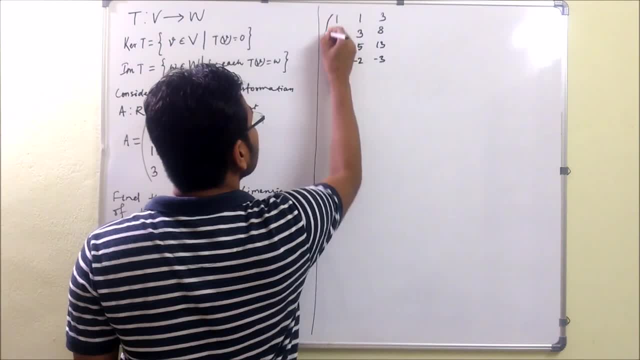 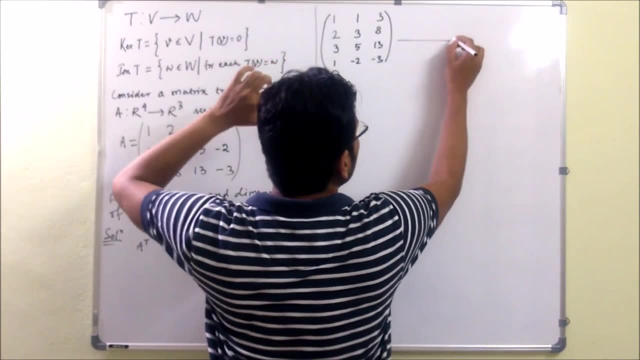 row is 1, minus 2, minus 3.. So how to reduce it into row equivalent form? So we have to apply Gauss-Helmson rule and we have to apply row reduction rule. So we have to first take: 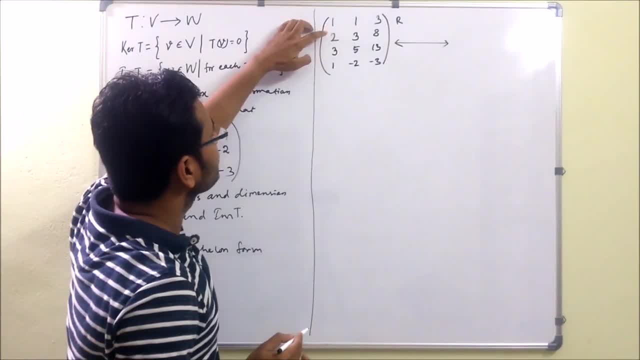 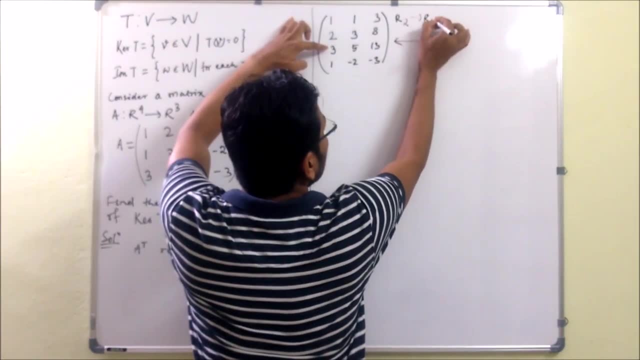 the first pivot element. First pivot element is this one. So below to that, this 3 entry, you have to make it 0.. How to make it 0?? So you have to convert row 2 as row 2, minus. 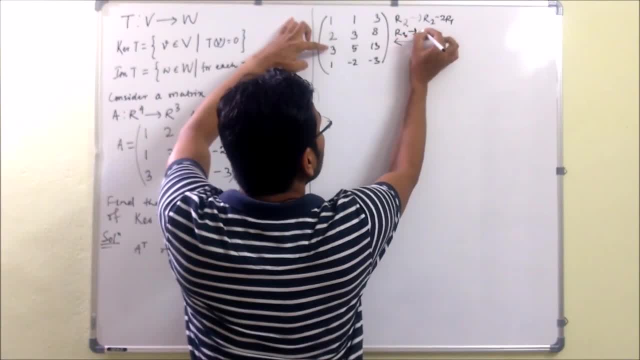 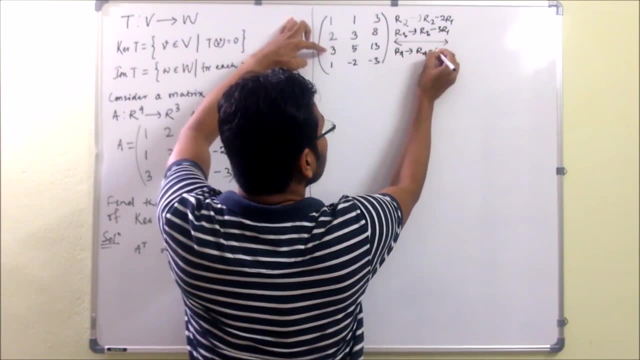 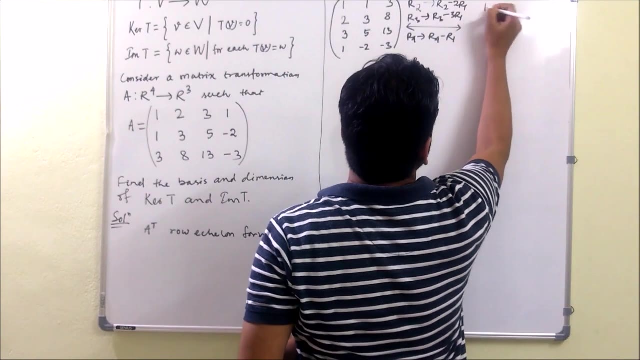 2, row 1.. Row 3 will be row 3, minus 3, row 1.. And row 4 will be row 4, minus row 1.. So if we do that, then what will happen? The first, so first row will be unchanged. That 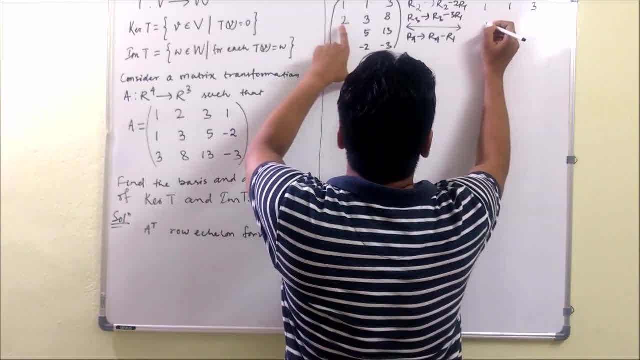 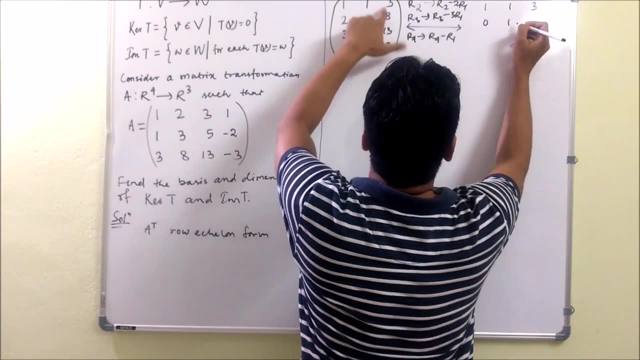 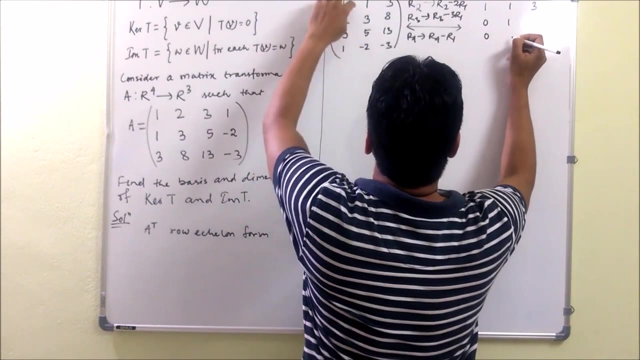 is 1, 1.. Second row will be this: 0, 3 minus 2,, 3 minus 2,, that is 1, 8 minus 6,, that is 2.. Then the second one is 0, 5 minus what? 3,, that is 2, 13 minus 9,, that is 4.. Then last will: 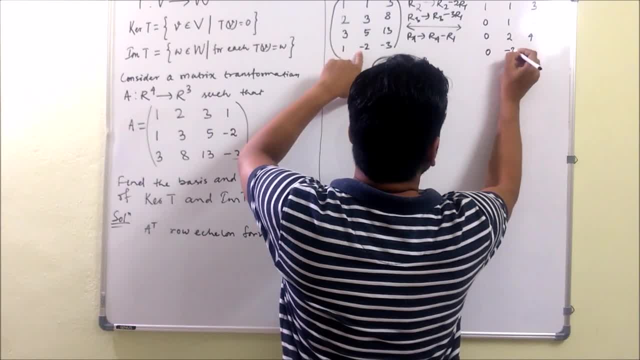 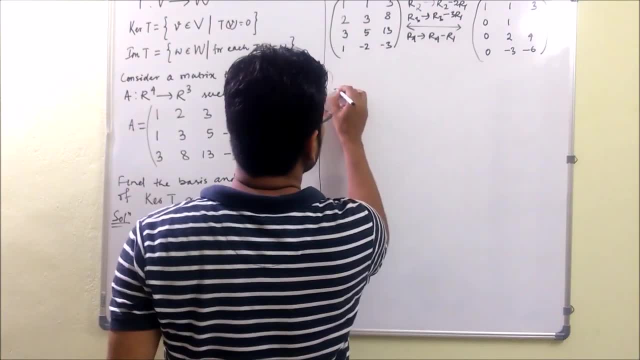 be 1, minus 1,, 0, minus 2, minus 1, minus 3, minus 3, minus 3, minus 6.. So you have to make it 0. So in this way we can get the second matrix. Now what to do Next? pivot. 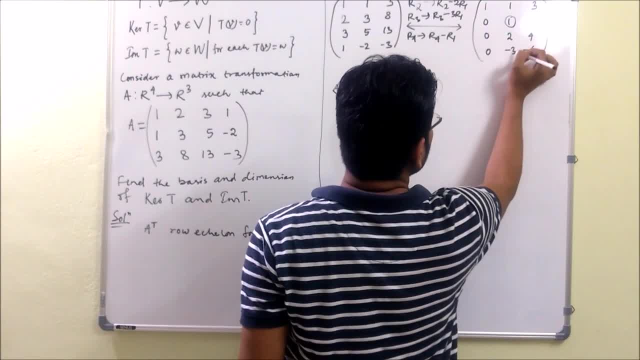 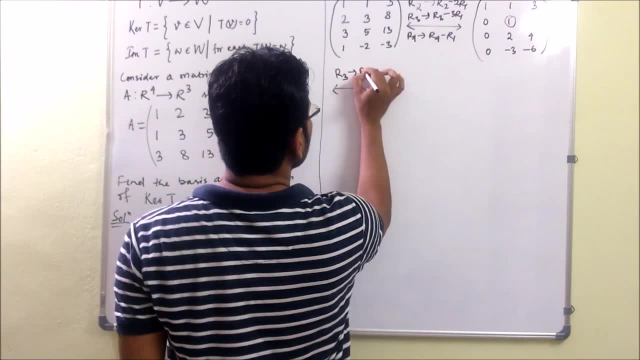 element is this one, So we have to make this 2 entry 0.. Below to this pivot element is this 2 element, so we have to make it 0.. So how to make it 0?? R3 will change to R3.